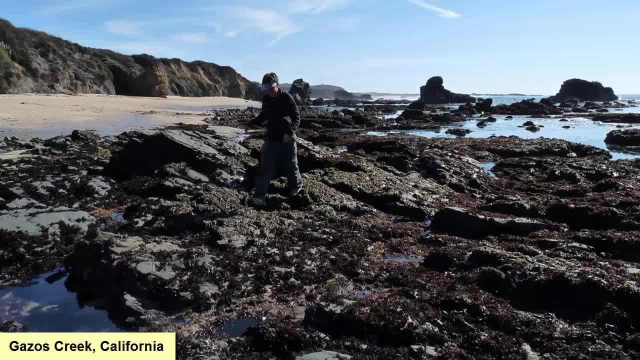 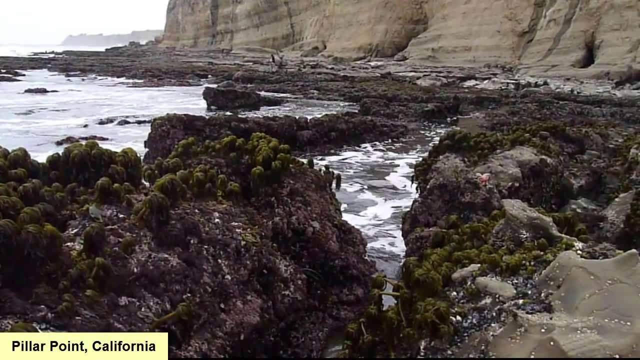 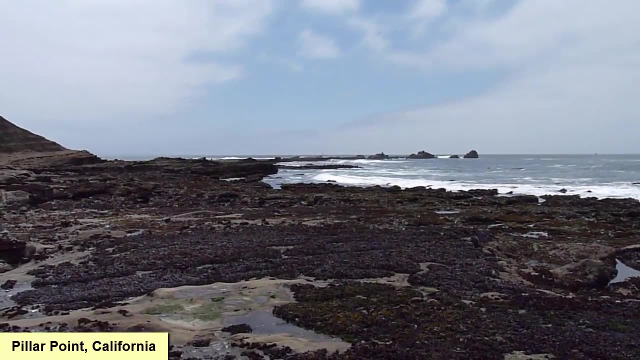 Now let's leave the nekton world and head down to the benthic world, starting with the shallowest parts of the ocean and the human entry point, the inner tidal zone. Remember: benthic means that an organism lives in or on the seafloor In the inner tidal. 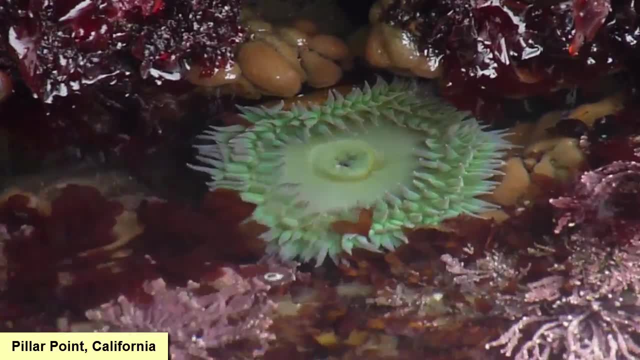 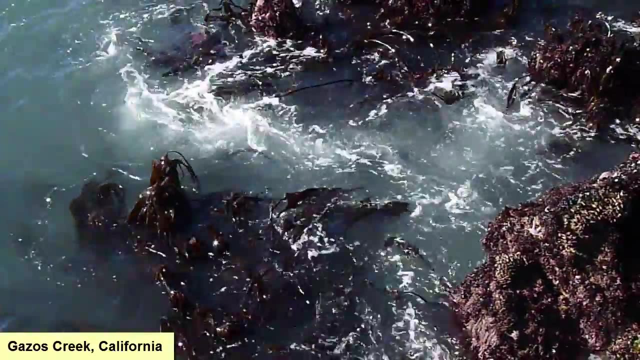 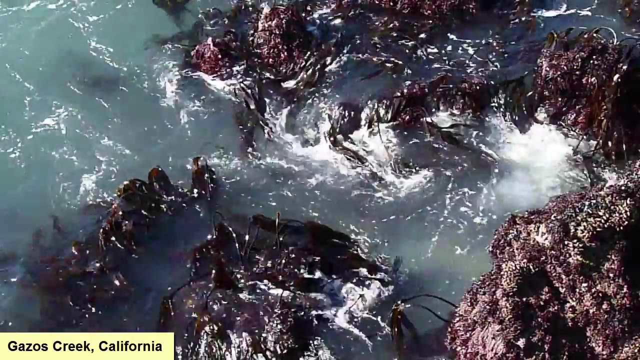 zone. life is buffeted continually by tidal currents, waves and changing environmental conditions, from high tide coverage to low tide exposure. Organisms that can survive this harsh environment must be able to combat these challenges and have found a number of clever adaptations for doing so. To prevent desiccation during low tide, animals have 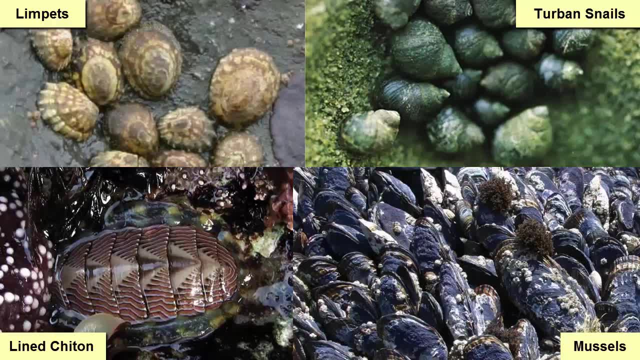 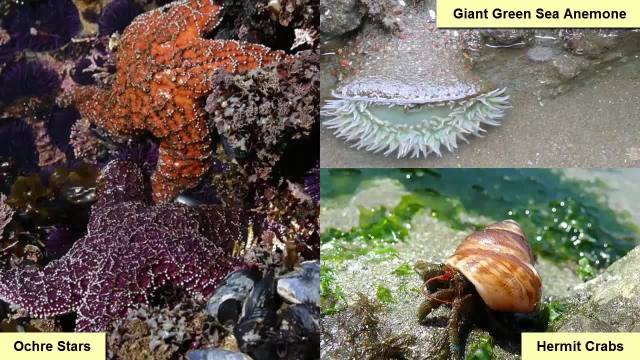 shells within which they can withdraw, like snails, limpets, mussels and hermit crabs, or they have thick skin, like sea stars and giant sea anemones. Some anemones stick light-colored sediment to their tentacles, then withdraw inside their bodies to prevent. 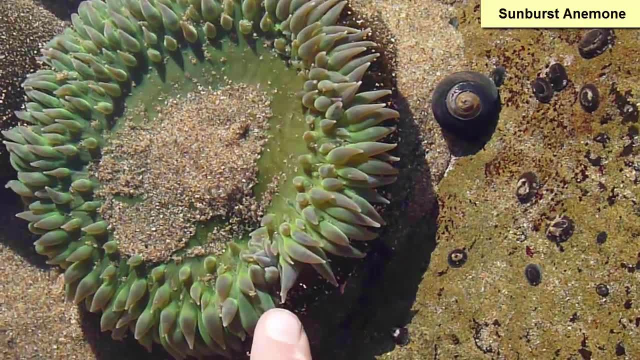 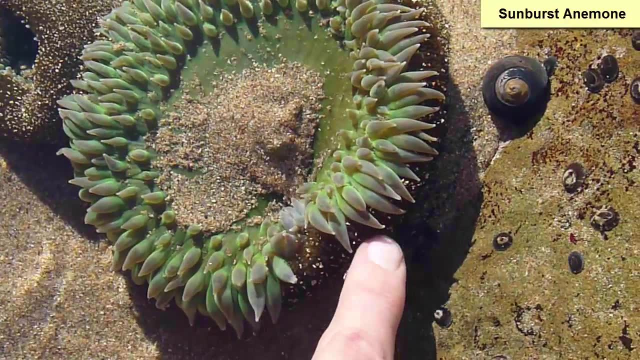 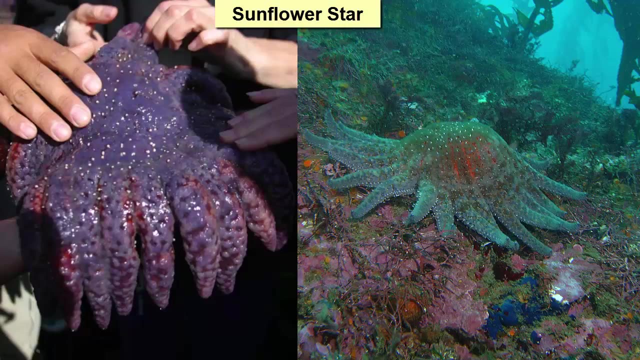 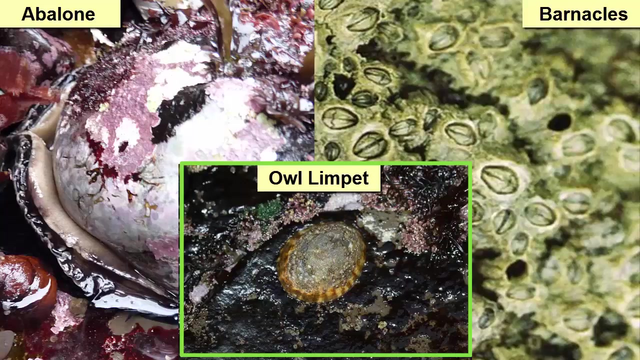 dryout and some sea stars emit a thick mucus coating on their outer surface to prevent dryout, To prevent being knocked around by high waves and currents. gastropods like abalone and limpets have strong feet that stick to the rocks. Barnacles attach their shells directly to 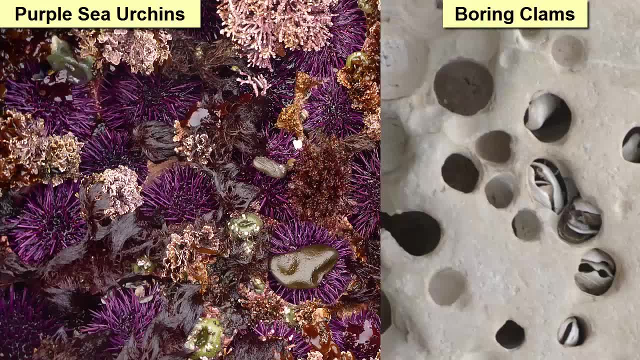 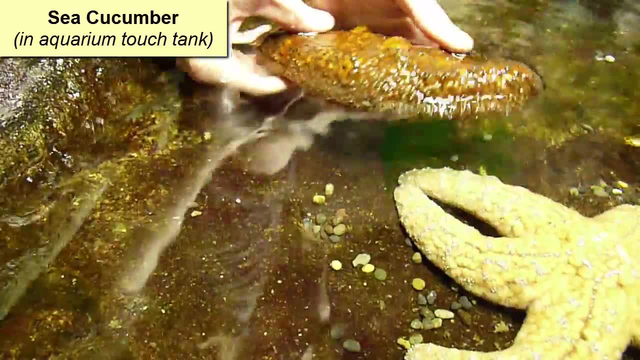 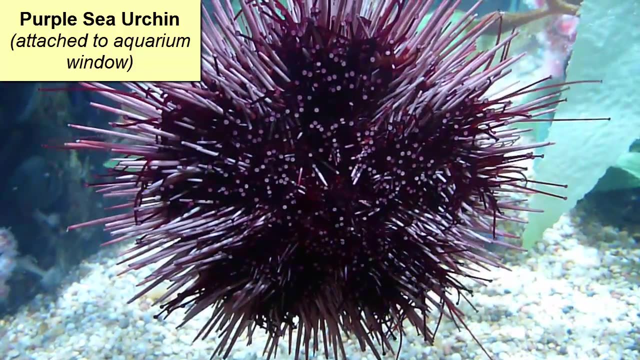 the rock, Sea urchins and boring clams carve out holes within which they nestle Sea stars. sea urchins and sea cucumbers have tube feet that stick strongly to the rocks thanks to their water vascular system, which creates high amounts of suction. Anyone who has ever 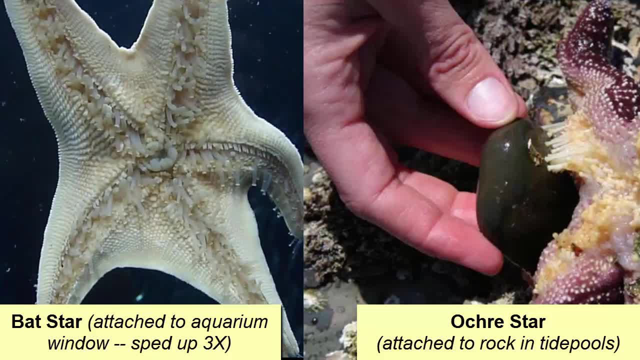 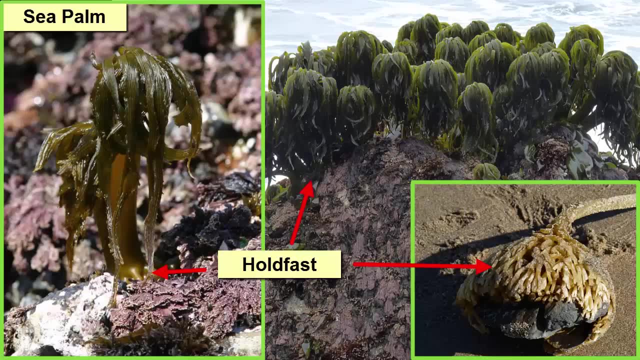 tried to pry a sea star off a rock knows how strongly they can attach Mussels. attach strong abyssal ViRIS threads to the rocks. Kelp attach themselves with holdfasts To handle the large range of predators that can arrive during high tide and low tide: anemone and. 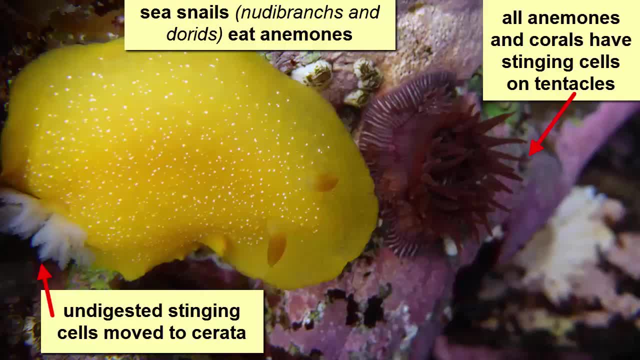 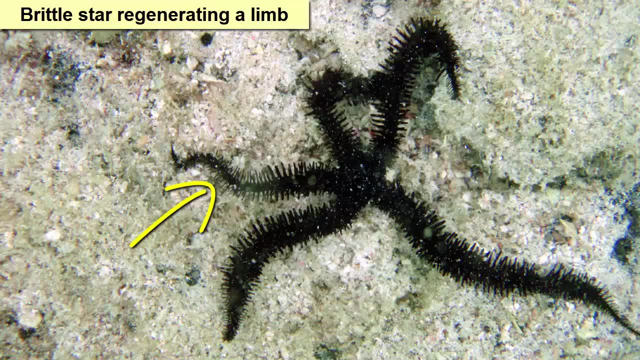 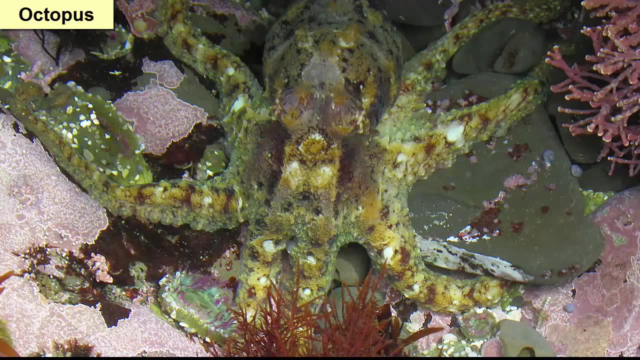 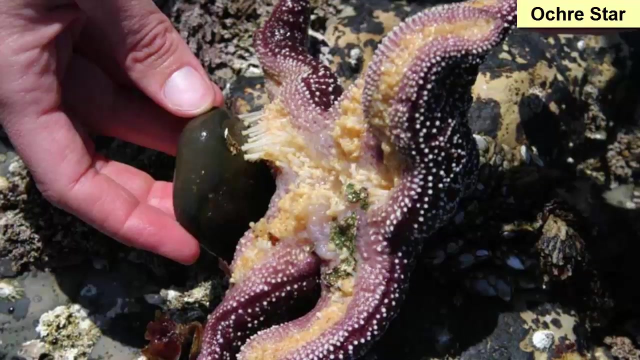 corals have stinging cells on their tentacles, 450 the same stinging cells for deterring their own predators. Sea stars can regenerate lost limbs. octopus can camouflage themselves perfectly to match their surroundings and can use ink to distract predators, And sea stars and mussels and others can clamp so tightly to the rock they are nearly impossible. 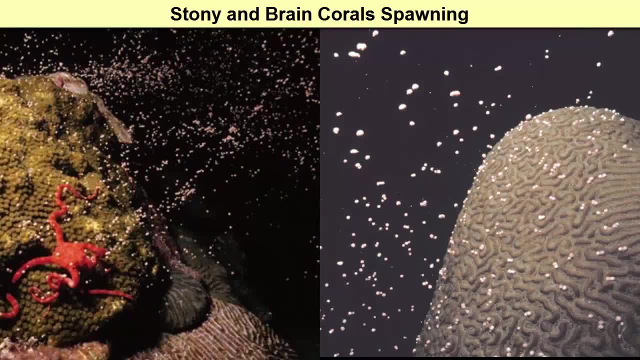 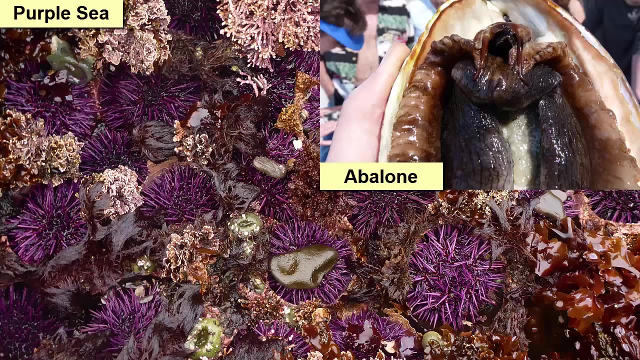 to pull off To handle the difficulty of finding a mate. sessile, permanently stuck, benthic intertidal organisms will release egg and sperm into the water column at the same time, like corals do, in the hopes that they will get together in the planktonic world. 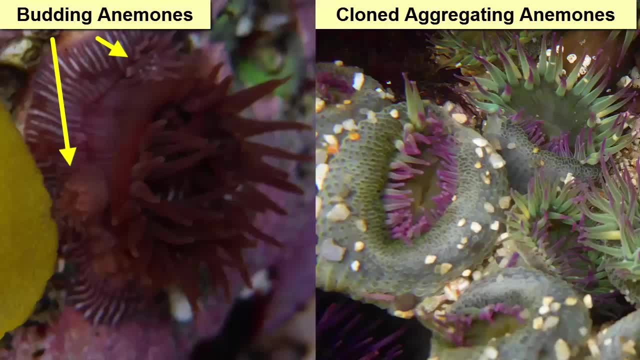 Abalone and sea urchins do the same. Many organisms such as anemones have a second method of reproduction- cloning- which they use most of the year to expand their populations. These anemones grow buds, which then migrate off their own bodies, take up residence next. 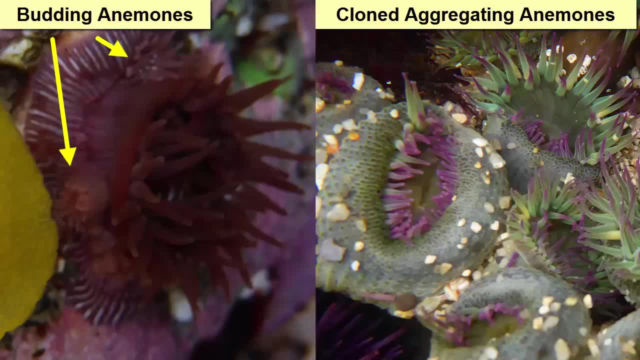 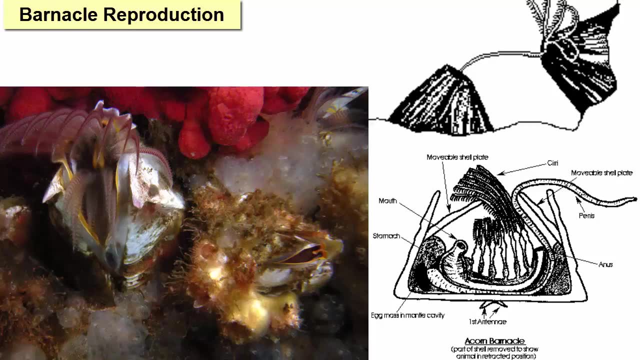 door and grow into a cloned version of the parent. Barnacles have a particularly interesting method of handling the difficulty in finding mates when you are permanently attached to a rock, The males have a very long penis which can reach out of the barnacle's own exoskeleton. 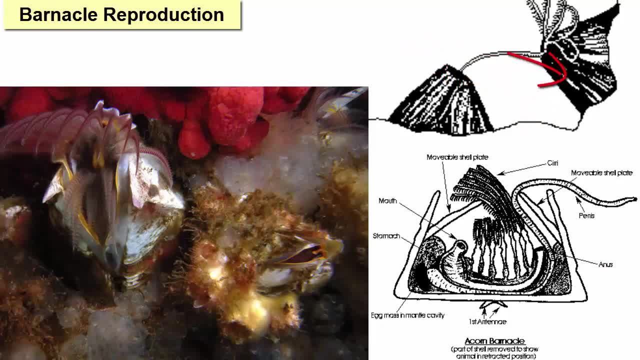 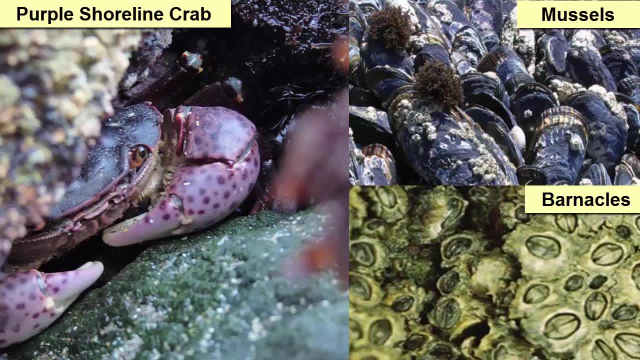 and reach outward in a large radius, probing and hunting for a ready-available female To handle the rapid changes in temperature, salinity, pH and oxygen levels that can occur during low tide when the rocks are exposed in freshwater rivers or in the ocean. the 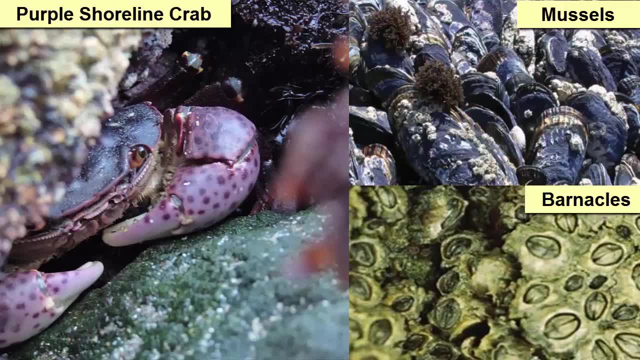 barnacles can reach out of the barnacle's own exoskeleton and reach outward in a large radius, probing and hunting for a ready-available female. Pollution and solar heating can radically change the surroundings. Organisms have shells in which they can retreat, such as barnacles. 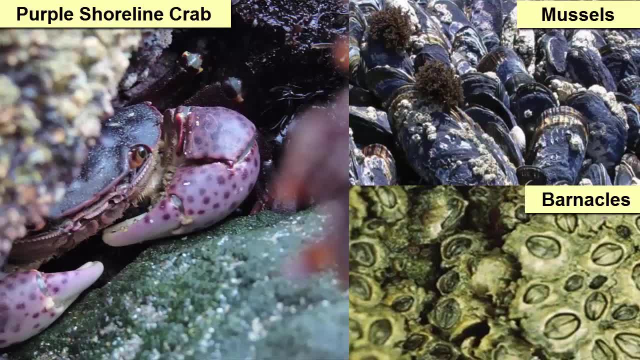 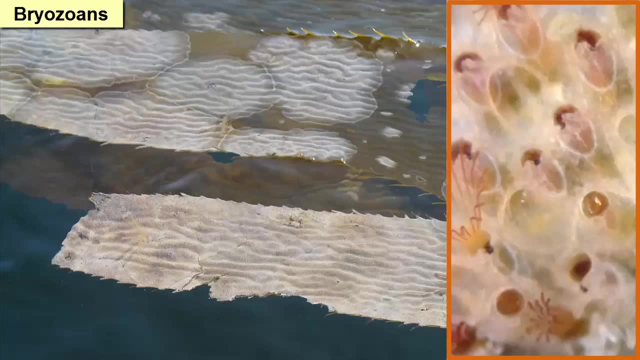 Most have adapted metabolisms that can handle these wide ranges and are thus urehaline and ure-thermal, and many can lie dormant and even mostly desiccated, with no damage, for up to 12 hours. Lastly, to handle the lack of abundant attachment sites, organisms have learned to live atop. 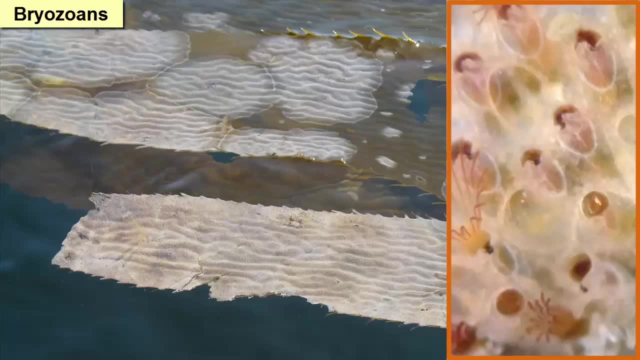 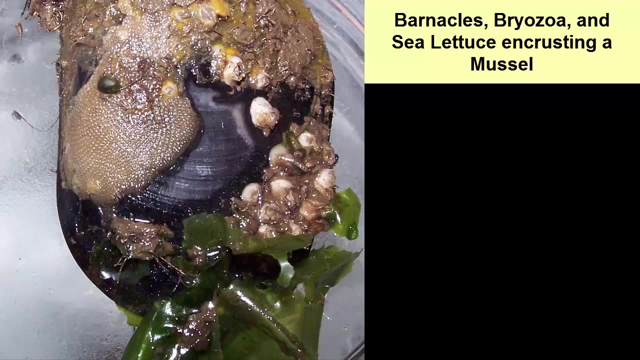 each other. Bryzoans cover the surfaces of kelp blades. Corals grow cloned colonies atop each other in branching and other ornate shapes And, as this image shows, mussel shells act as surfaces on which barnacles, bryzoans, tunicates, sponges and sea lettuce can grow. 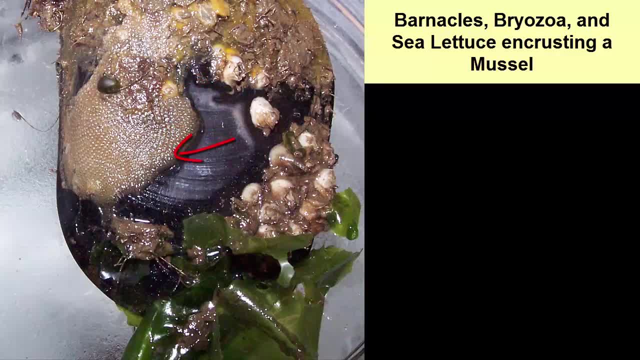 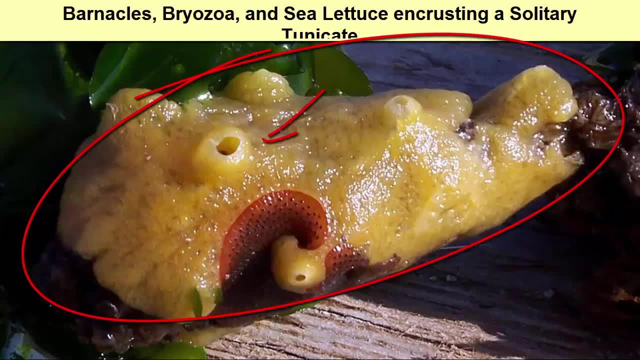 In this picture there's a barnacle atop a bryzoan colony. atop a mussel shell, As this other image shows, we have a large solitary stock tunicate covered by an encrusting sponge, which is itself covered by these red bryzoans. 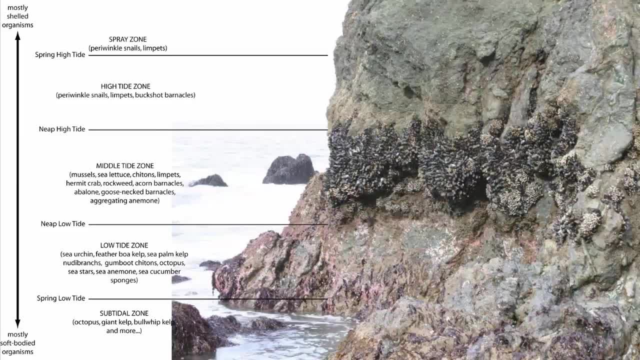 Due to these many intertidal challenges and adaptations, the rocky intertidal shorelines typically show vertical zonation, which means that organisms that are uniquely adapted to survive in one of the many zones will thrive in those zones and be found only there. 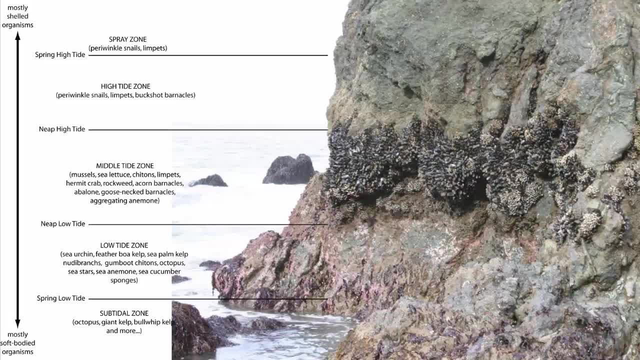 In fact, they will likely competitively exclude other species from those zones. Competitive exclusion is a process where a favored species can out-compete other species for resources, reducing the diversity of a community. This image shows many examples of vertical zonation and competitive exclusion. 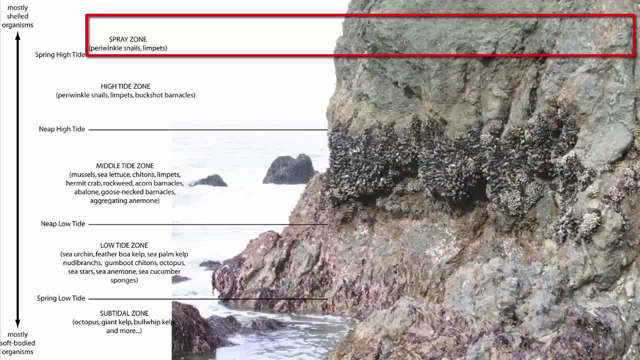 The spray zone is the zone that is rarely ever covered by water, but will be exposed to wave spray during high tides on stormy days. Organisms that are most competitive in this zone can handle small amounts of seawater and plenty of above-water exposure. 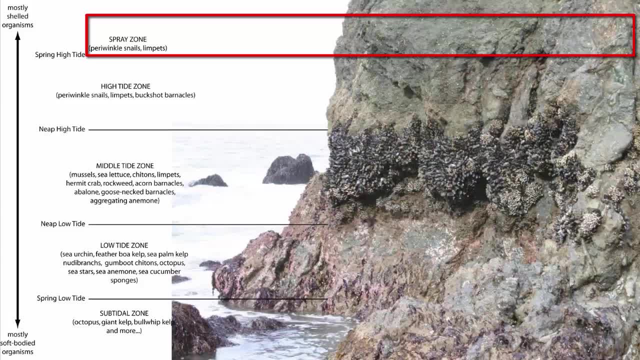 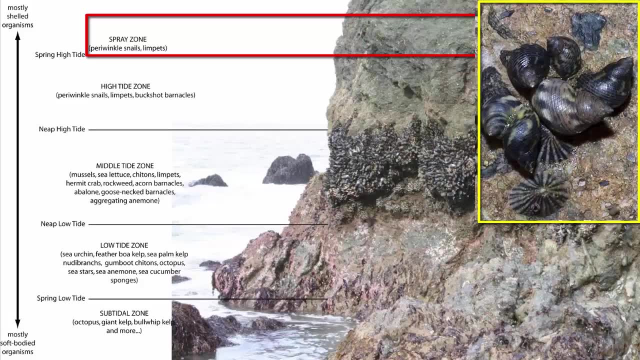 They are unique from other lichens, but they can also be found in other species. They are unique from other land organisms in that they can handle high amounts of salt and occasional submerging. Examples of organisms who thrive in this zone are limpets and periwinkle snails. 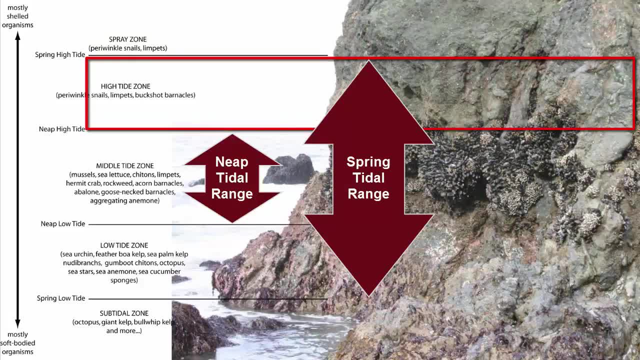 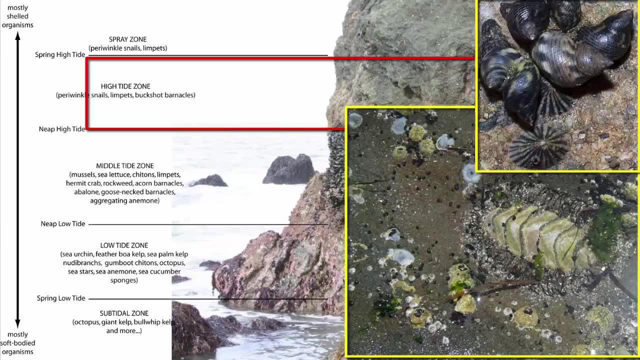 The high tide zone sits between the neap high tide and the spring high tide. That means it will be covered at most only a few hours a day and then only every two weeks. Organisms in this zone include again the limpets, the periwinkle snails. 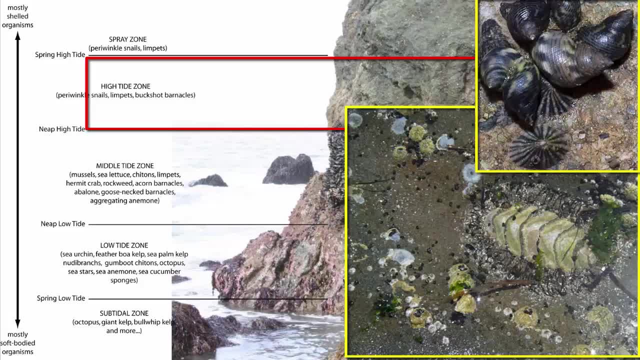 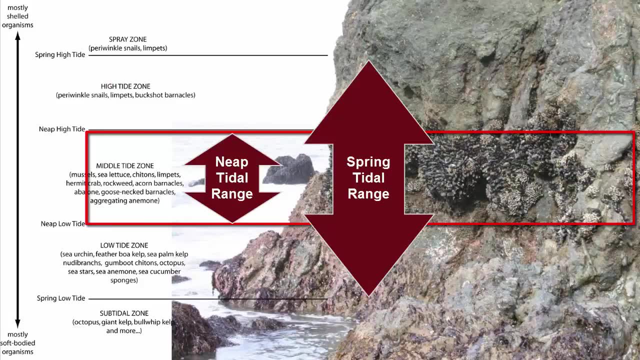 but also buckshot barnacles and chitons. The middle tidal zone is the region of the inner tidal that is always alternately covered and uncovered each day. The top of the middle tide zone is the neap high tide. The bottom of the middle tide zone is the neap low tide. 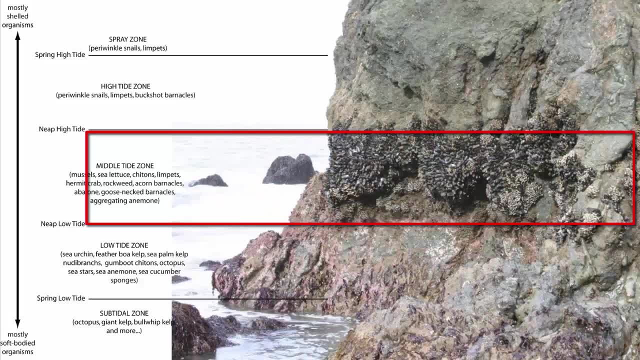 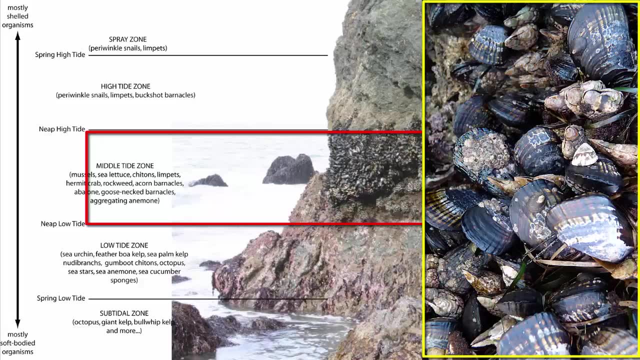 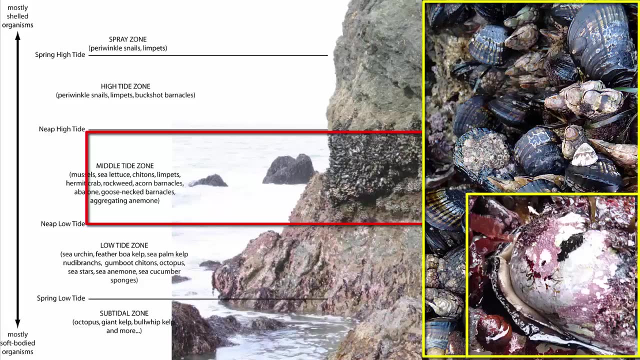 Organisms in this zone must be able to handle the most consistent alternation of wet and dry. Muscles are the most competitive at handling the top of this zone zone, along with sea lettuce, Abalone, like the middle and lowest parts of this zone, as do acorn barnacles, gooseneck. 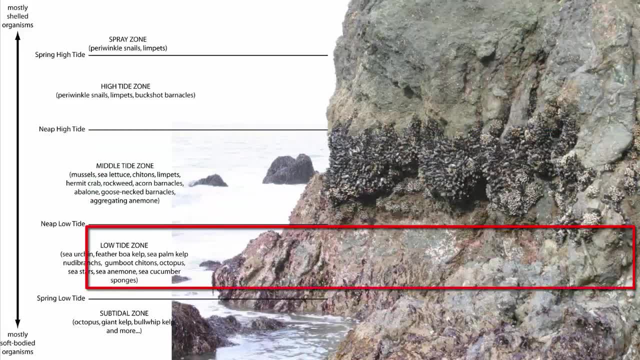 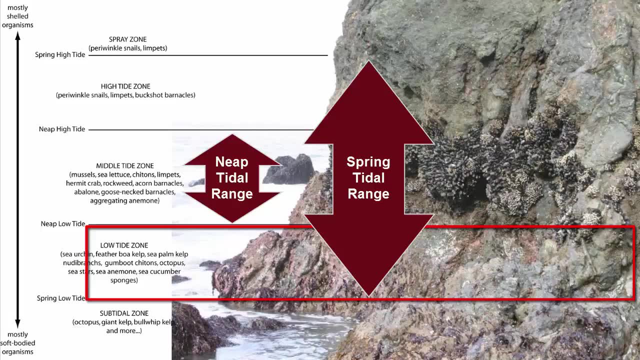 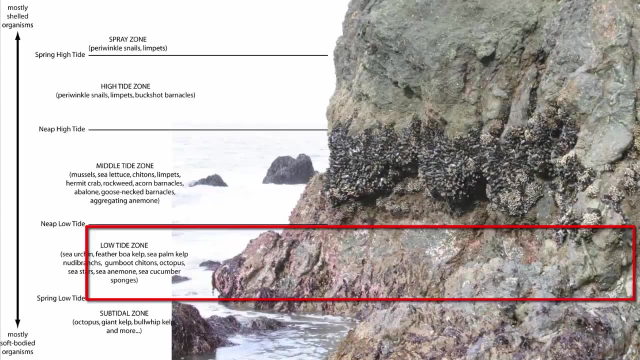 barnacles and hermit crabs. The low tide zone is uncovered only during the lowest low tides. It is completely uncovered during low spring tides and never uncovered during low neap tides. Competitive organisms in this zone can handle mostly being submerged and very limited times.